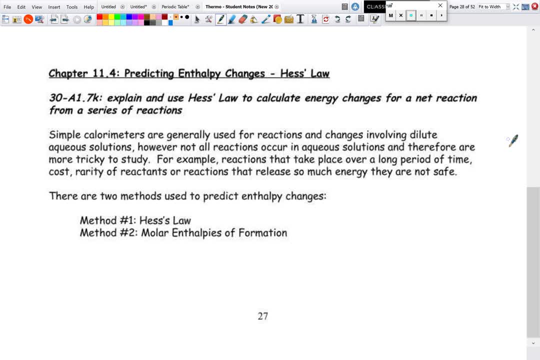 calorimetry experiments. we know that when we do stuff in like a coffee cup calorimeter where stuff are in aqueous solutions, we get really good results. because water has such a high specific heat capacity, it's not going to lose a lot of energy to the calorimeter and everything just. 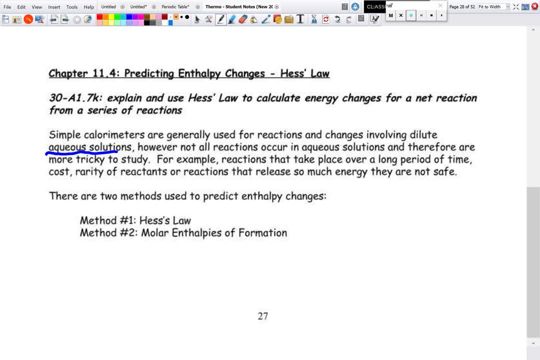 works wonderfully. However, not all reactions are going to occur in aqueous solutions and are trickier to study, So some reactions take a long period of time, it may cost too much, reactants might be extremely rare or they release way too much energy and it's not safe. So when this happens, 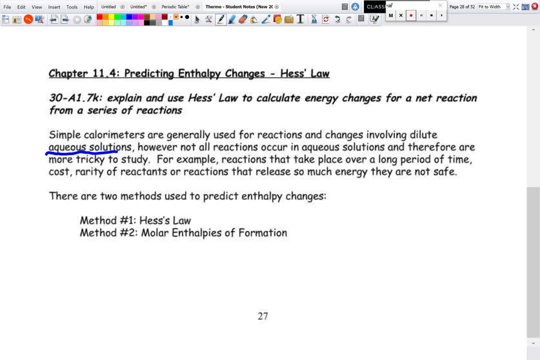 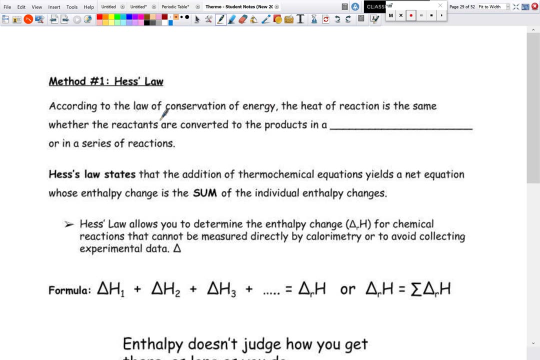 we're going to use two different methods to predict enthalpy changes and also try to find molar enthalpy for certain objects or chemicals. The first one we're going to look at is Hess's law. Now, Hess's law states that, according to the law, 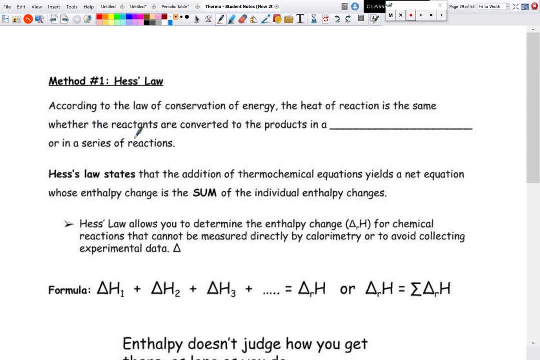 of conservation of energy. the heat of a reaction is the same whether the reactants are converted into products in a single step or a series of reactions. Because when we think about, enthalpy is just the or enthalpy change is just the change in potential energy. 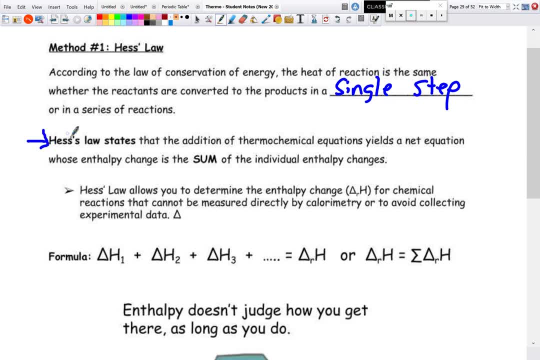 So what we're going to do is we're going to look at a series of reactions, and what we're going to really look at is a series of reactions, and what we're going to look at is a series of reactions. So this is where Hess's law comes in. It makes use of that idea and it states that the addition of our 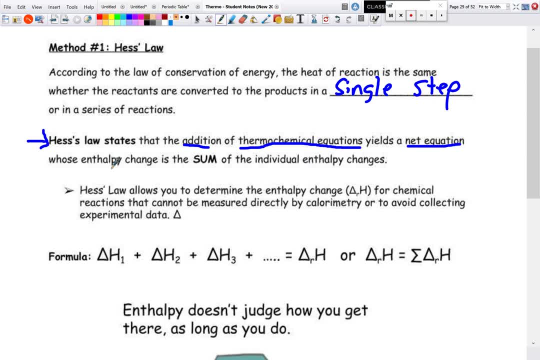 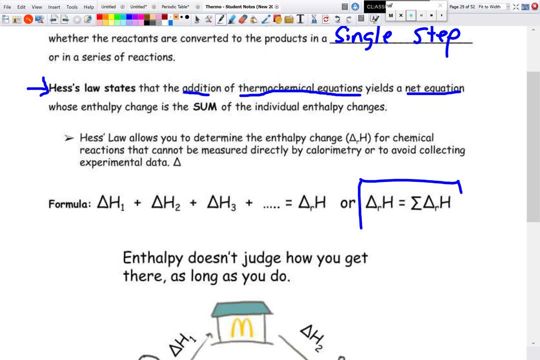 thermochemical equations yields a net equation whose enthalpy change is the sum of the individual enthalpy changes. Now that just translates into this. So remember to change in enthalpy is equal to the sum of all the enthalpy changes in a reaction, and remember this sigma is the sum of for. 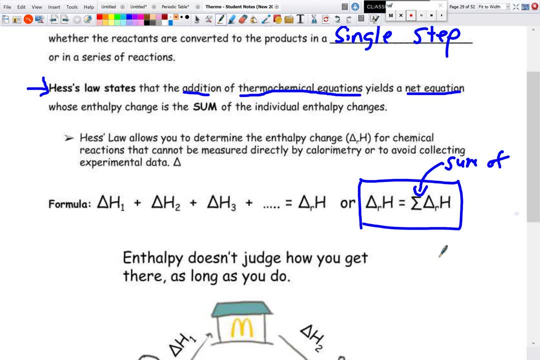 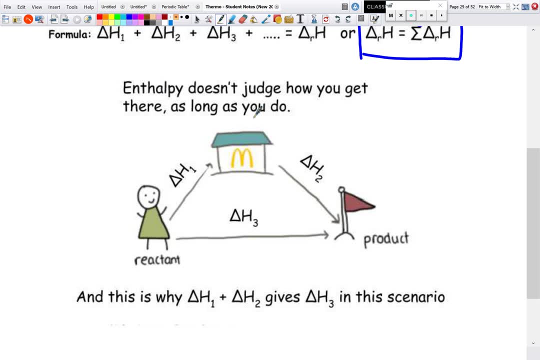 those who haven't seen that math for a while. So this little picture right here, this is just one that I came across, and it is true So enthalpy. doesn't judge how you get there, as long as you do. So when we look at this right here, we have our reactants on one side and our products. 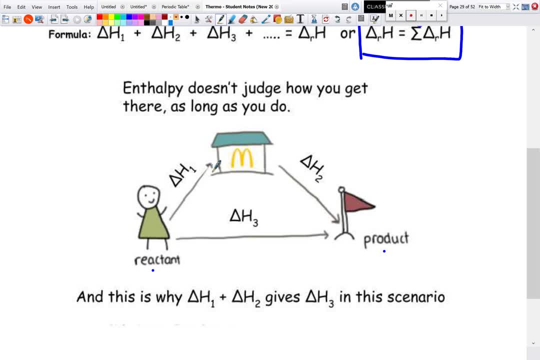 on the other, If this person decides to make a side trip over here. so this associated enthalpy change one goes to McDonald's, boom comes back enthalpy change two. well, it doesn't matter, At the end of the day they're arriving as a product. 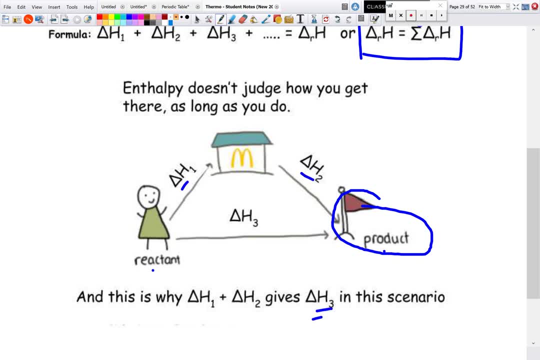 So this is why delta H1 plus delta H2 will give us delta H3, and that's going to be true for all of our reactions. So it doesn't matter how many steps it takes, as long as we get there, that's it. 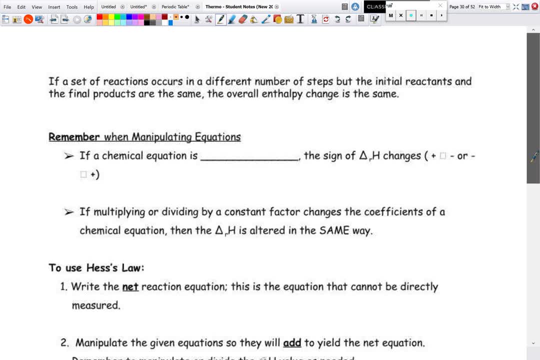 Now. I know that's going to be a little confusing right now. So when we get there, don't worry, we'll kind of see this a little more, and when we get to our first example, it'll definitely make a lot more sense. 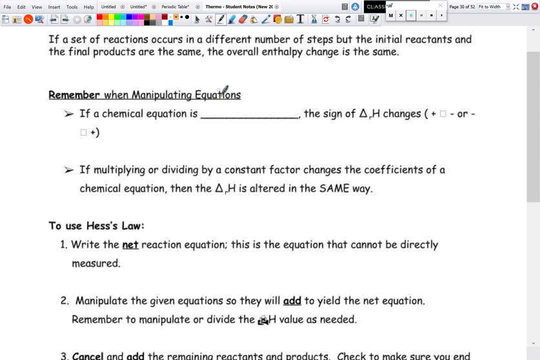 Now we're going to have to manipulate equations and add them together, right, Because that's what Hess's law is all about, Is adding, Adding, Adding, Adding, Adding equations together. So when we add them together, we get a net equation. 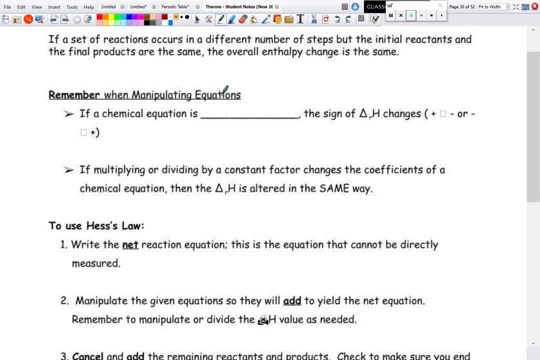 Now we've seen this in net ionic equations, where we added our ionic equation and we simplified it down to our net ionic. So we've seen that before: where we add stuff together, we cancel things out. Now one thing that we haven't really seen before is that if a chemical equation is reversed, 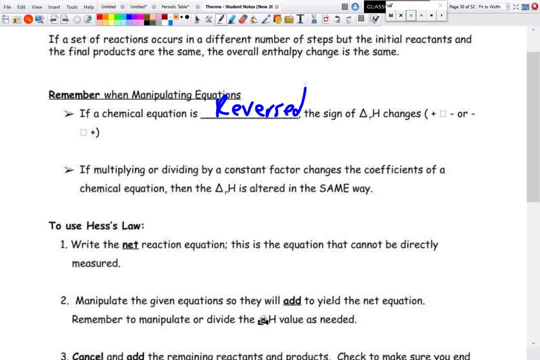 Now we've kind of seen it, we kind of haven't, But I'm just going to show you. I'm just going to give you an example here now in a sec. So if a chemical change is reversed, the sign changes. So that means, if it's the delta H is a positive, it'll turn to a negative. 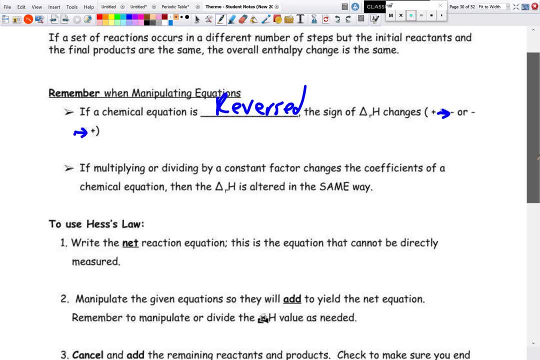 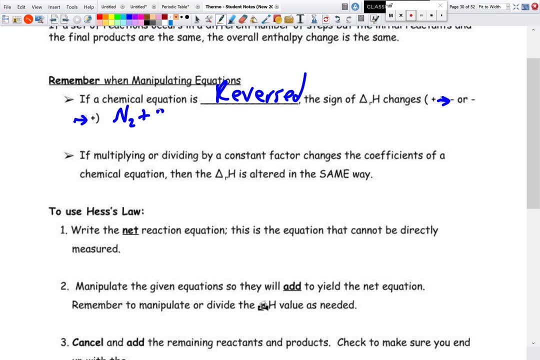 Or if it was a negative, it's going to turn to a positive. Now, an example of this is that one reaction, if we know it's exothermic. So N2 plus 3H2 produces 2NH3 and delta, and this will be a formation. 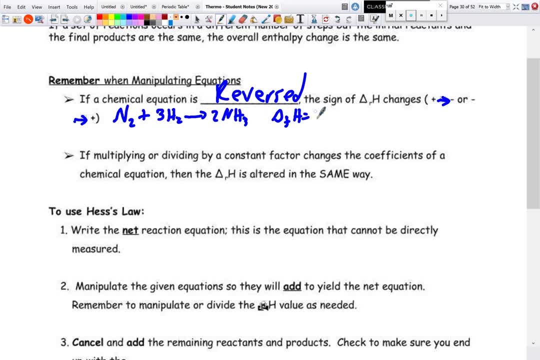 So if we know that the second reaction is equal to- I can't remember the actual number, I think it's negative 97.5 kilojoules. Now, this is a formation reaction. We have plus, element produces compound. Now, we kind of made this connection as well when we were doing our review. is that a decomposition? 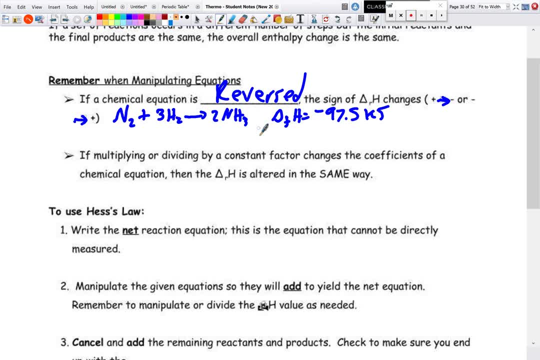 reaction is when we start with a compound and we produce the elements. So if we were to decompose ammonia- I'm going to write this in another color, though, just so it's a little different- So if we're to decompose ammonia, so start with 2NH3 and decompose it into nitrogen and 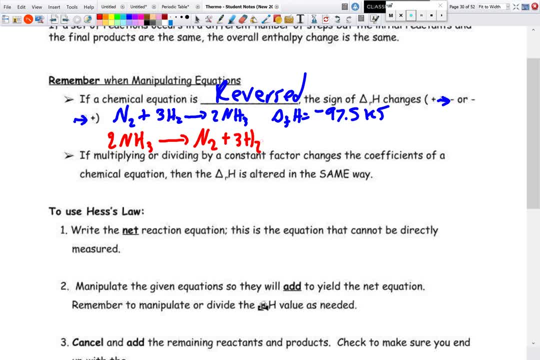 hydrogen. now notice this is like literally the exact same reaction. it's just written in reverse. So if we were to do that- reverse a reaction- well, we would reverse a sign. So if the formation is exothermic, the decomposition is going to be endothermic and we have the 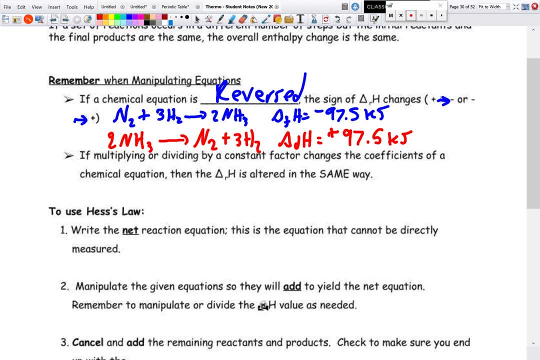 exact same numerical value, it's just the signs are different. Now we've seen this as well when we looked at photosynthesis and cellular respiration in one of our examples back a few pages ago. So if you go back, I think that was the example after communicating enthalpy changes, where 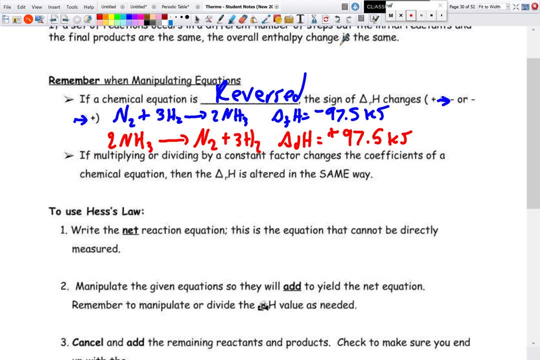 we wrote the three methods of communicating enthalpy change for photosynthesis and cellular respiration. So they're the exact same number of energy because they're literally reverse equations of each other. Now also, we've seen examples like this as well, where we can multiply or divide by a. 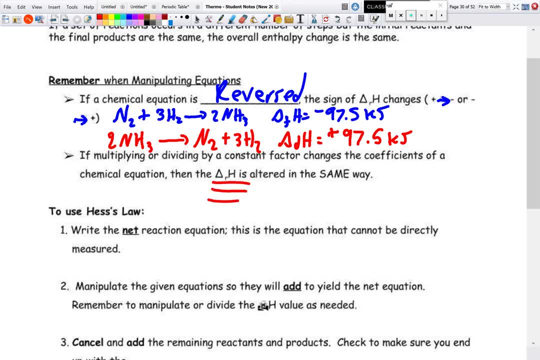 constant factor, and if we do that, the delta H value is altered in the same way. So if we multiply an equation by 2, we also need to multiply the enthalpy by 2.. Now to use Hessel's law. there are a few rules here. 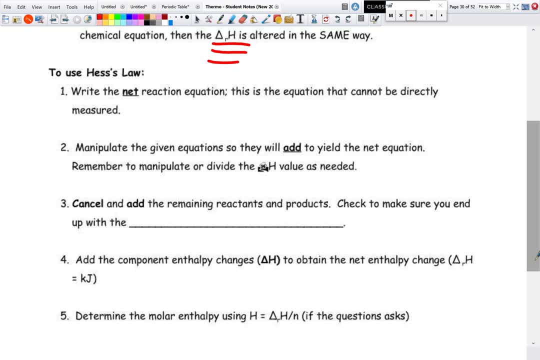 So we're just going to go over the rules and if it doesn't really make sense, it will when we start getting examples. So first of all we need to write the net reaction of the equation. if it's not given Now, normally this is the equation that can't be directly measured. 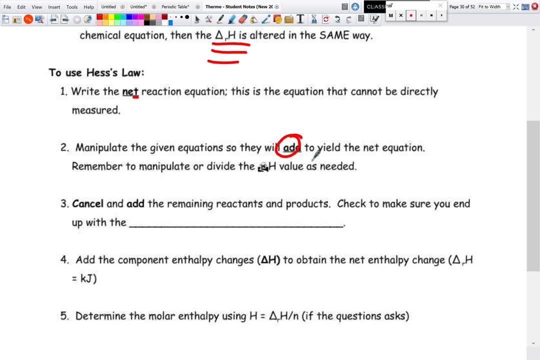 Next, we're going to manipulate all the given equations. so when they add up, they yield the net equation we wrote out in step 1.. And we also remember to manipulate our delta H values as well. Now, once we do our manipulation, we're going to cancel and add all the remaining reactants. 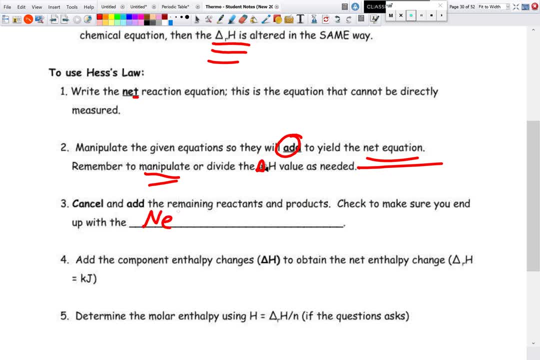 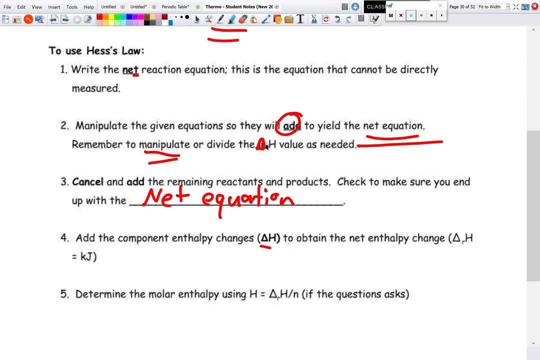 and products, Just to check, to make sure We end up with the net equation. So this is just double checking our work, making sure that we actually manipulated everything correctly. Now, once we have all that, we are going to add all of our enthalpy values together. 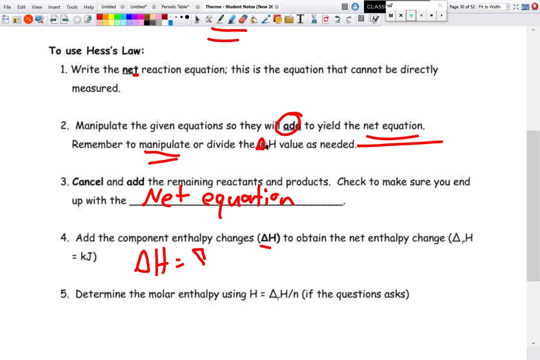 And that's where we go. delta H for the reaction is going to equal the sum of all of the smaller reactions. And step 5 is optional, but you have to read the question just in case it asks for the molar enthalpy using this equation: 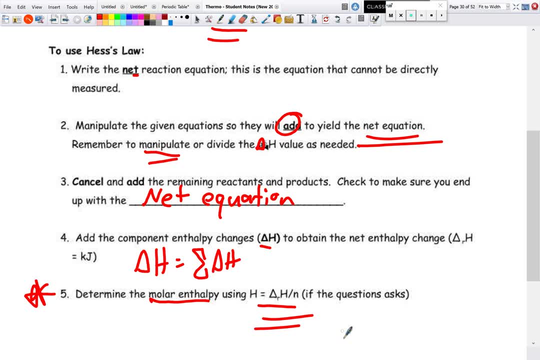 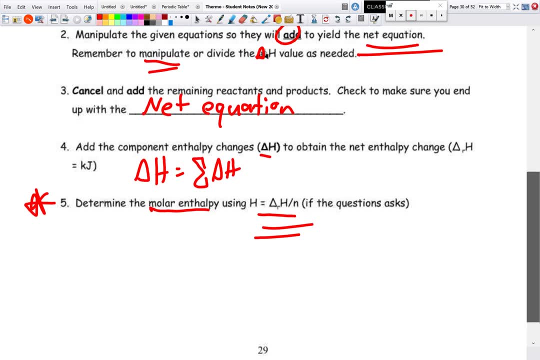 And that's of course if the question asks. So, like I said, we're going to look at our first example and then hopefully, all these will make a little more sense. Now I know, on stuff that's printed out, we have example 1 down here and there's an iron. 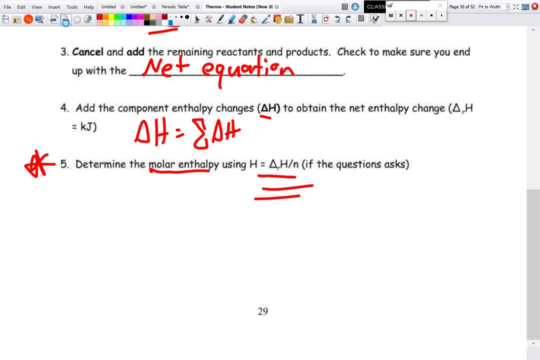 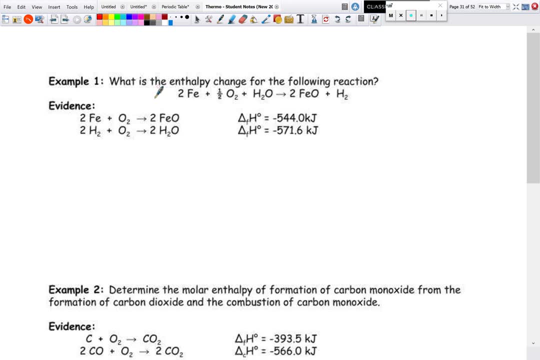 one, but for some reason the copy I'm using is different. Should be the exact same book. I don't know what's going on, but anyway this is what it should read. So if yours is a little different, just write this equation above. 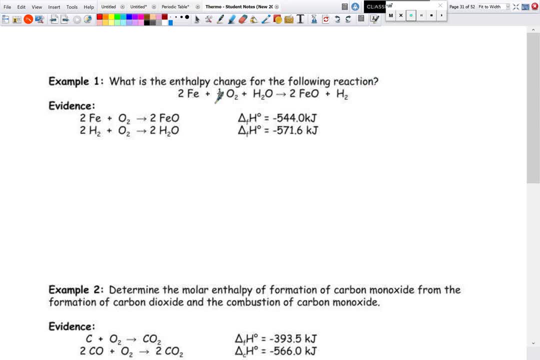 So it says: what is the enthalpy change for this following reaction? We have two irons, It's plus half. an oxygen plus water produces iron oxide and hydrogen. And we need to get this equation, this net from our two given equations, right here. 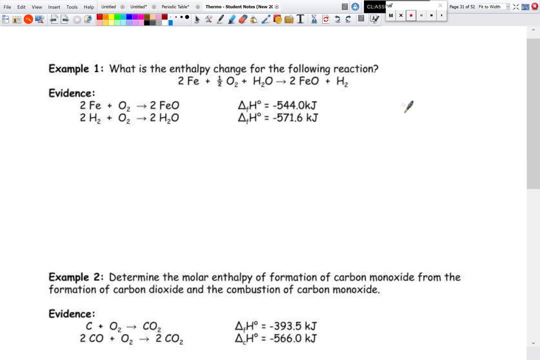 Now, when you're doing Hess's law, you want to look for unique elements or compounds in our net equation and then try to manipulate our given equation so that they are on the correct side of the equation, and then also with the correct coefficient. So what I mean? 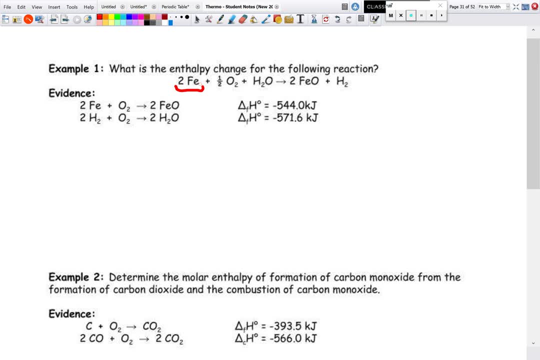 When we look at iron here. so we need to have iron as a reactant in my net equation. Now, out of my given equations here, equation one is the only one with iron, So therefore, if I use this one, this is: this is how I can get iron into my net equation. 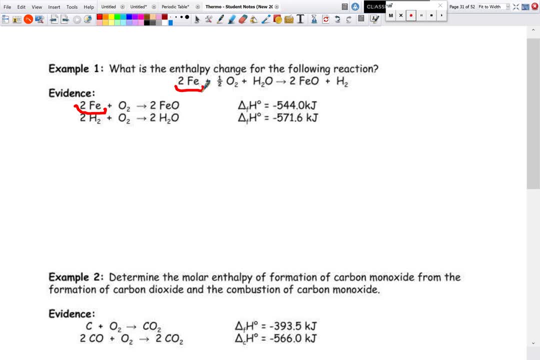 Now, here I can see: iron has a coefficient of two and it's a reactant. in my given equation, Iron has a coefficient of two. So they match right. Two and two They match And it is a reactant. So, based on that information, because iron is on the correct side of this correct side, 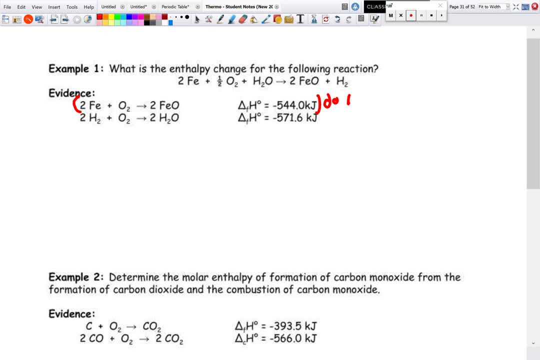 of the equation and it has a correct coefficient. we are going to do nothing to this equation Now, just because I I'm doing nothing to it. I like to rewrite everything in my own writing, just so I can add them up later. So I'm just going to take this: 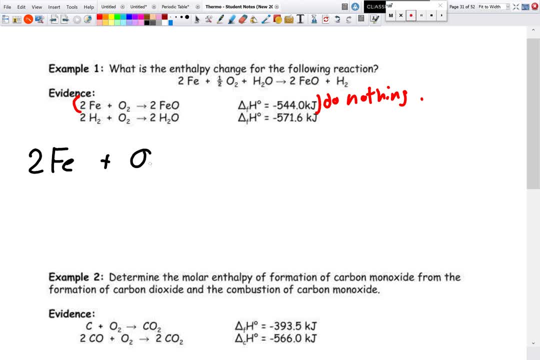 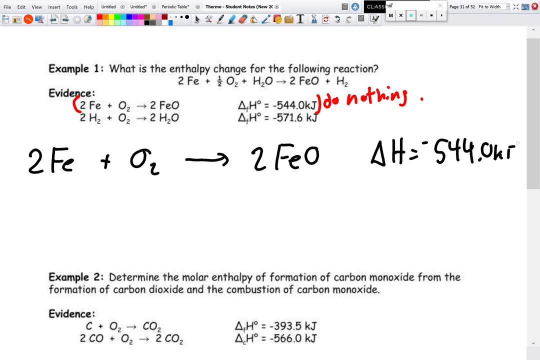 Now I just like to do that, write it in my own writing, because I want to make sure, if I have to manipulate this one, I get to put the arrows together and you know it'll. everything will look nice, but you'll see when I start adding stuff together. 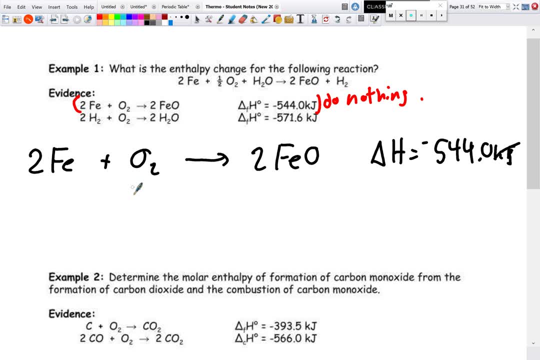 So you don't need to do this, um, if you don't want to. So once I do that, I'm going to then scratch- This is great- this out, because i've done manipulating it. technically. i've done nothing, but i don't want. 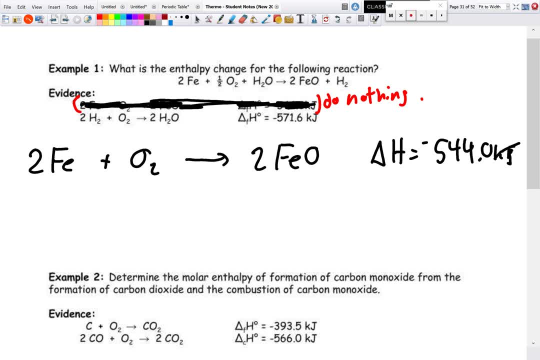 to see it anymore, right, because if i see it, i'm i might get confused, so i scratch it out now. my next one: if we look at our net equation again, now i'm just going to look for hydrogen, because hydrogen is unique here and it's unique down here. right, i could do oxygen or water as well. anyway, hydrogen. 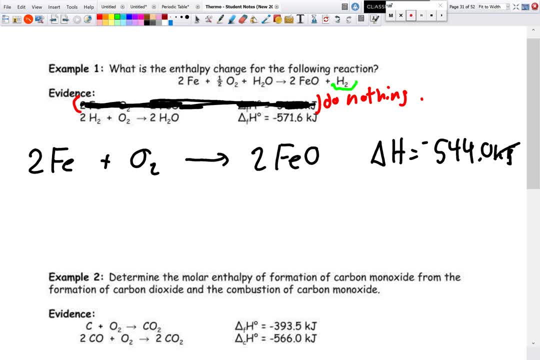 just kind of jumped out at me. so when we look at hydrogen over here, hydrogen is a product and the coefficient in front is one. on this equation, though, hydrogen is a reactant and the coefficient is two. so it's on the wrong side and it has the wrong coefficient. so i'm going to take this. 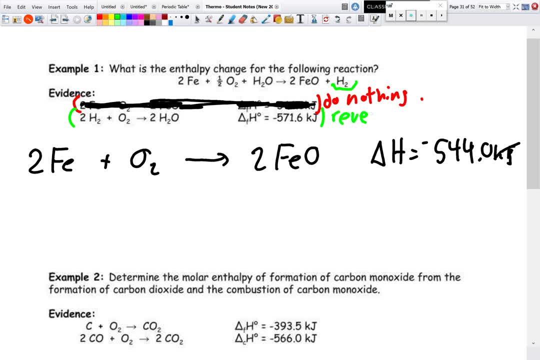 equation. first of all, i want to reverse it, just because if i reverse it now, i'm going to bring hydrogen over to the product side, which i want, but i'm also going to divide by two, so so so I can get the correct coefficients, meaning that 2 is going to turn into 1, this is going. 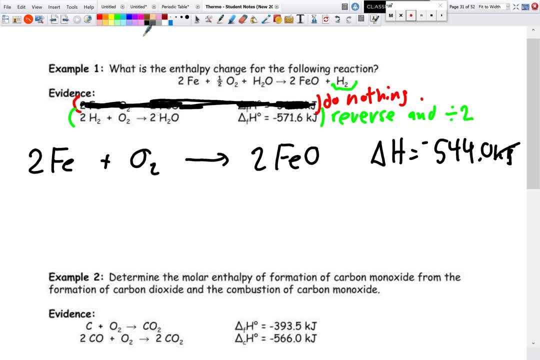 to turn into 1 half and this will turn into 1.. So now my new equation is this: reversed, so I'm going to have H2O on this side and I'm going to get H2 plus 1 half O2, right, remember, because I also divided everything by 2, and 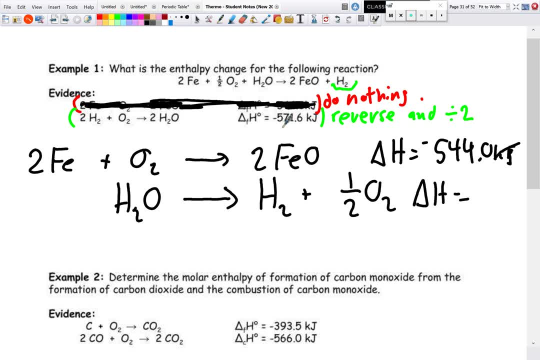 delta H. now that means I need to reverse this, so it's going to turn into a positive and I need to divide 571.6 by 2, and I get negative 258.2 kilojoules done. Now we are going to check to make sure that – oh sorry, I forgot one thing after I. 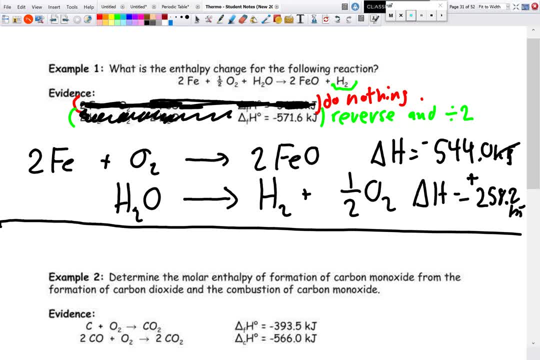 manipulate it, I'm going to fix it, I'm going to scratch it out so it does not come back and confuse me later. So these are my two equations I have manipulated. Now I'm going to add them together to see if I get my net. 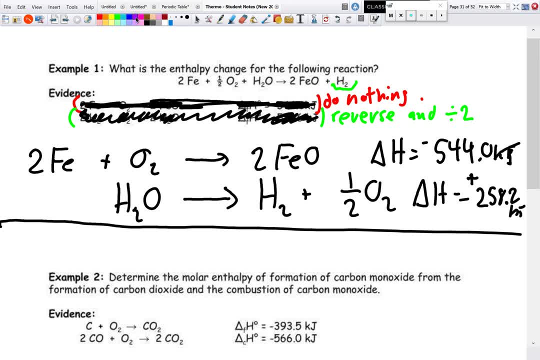 So we are going to – if we have the same component or element on the exact same side of the equation, we're going to add together. if they're on opposites, they're going to cancel. Now, when we look at – we have iron as a reactant over here. there's no irons as. 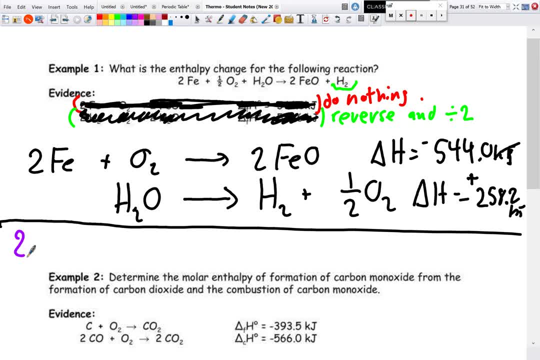 a product. there's no more irons as a reactant, So our 2Fe2.. Fe is going to get dropped down. Same thing with our water, because we have water right here as a reactant. there's no other water as reactant, so there's nothing to add to it. but there's no water. 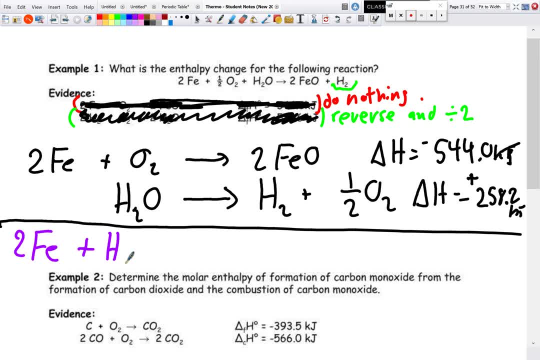 over here as products to cancel out. So my H2O, Now my oxygen. we will notice even though the coefficient isn't there. there should be a coefficient of 1 in front of this oxygen. I don't like writing 1 because that just looks like 10, right. 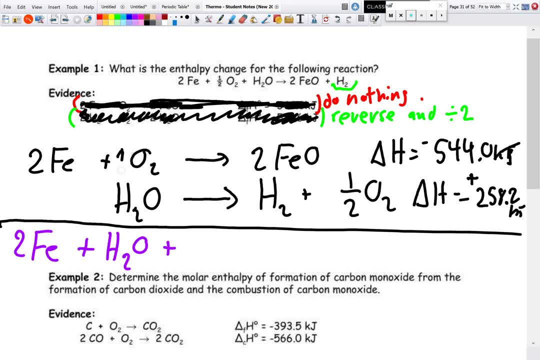 But anyway, we have 1 oxygen Okay. Now on this side, however, notice how we have half an oxygen Now. we've seen canceling before, where the – basically everything will cancel out, But because we have half an oxygen here and only 1 here, obviously half is less, so this: 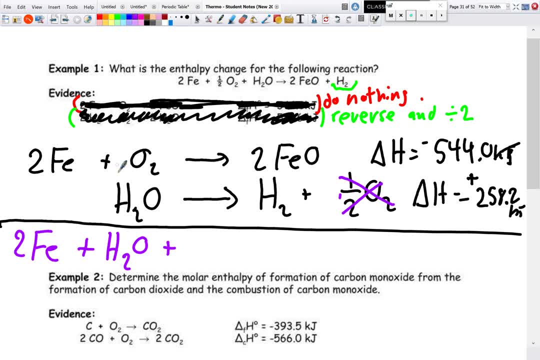 oxygen is going to get completely used up. Now the new coefficient from this oxygen. I need to do a little bit of math. It's normally a coefficient of 1.. Now, because oxygen is on the other side, right, we're going to subtract the half, that's. 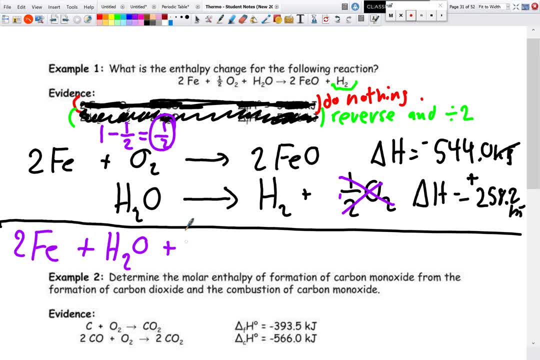 what it's losing And equal 1 half. So this 1 half is going to get in front of this oxygen and we bring it down to 1 half O2.. Then we go arrow- Same thing. We see iron oxide. nothing can cancel it with. 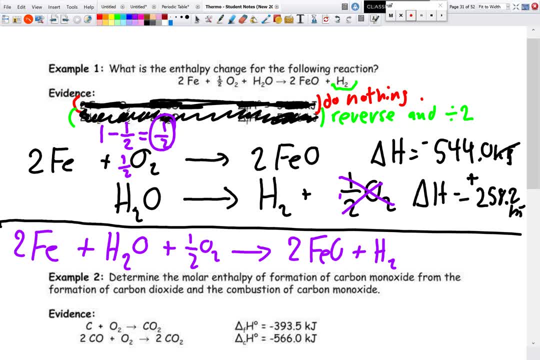 So 2 FeO and then plus H2.. So you'll notice this is equal to this. So my net. I like to give myself a little check mark, knowing that they're the same. Now I'm going to pull up something over here. 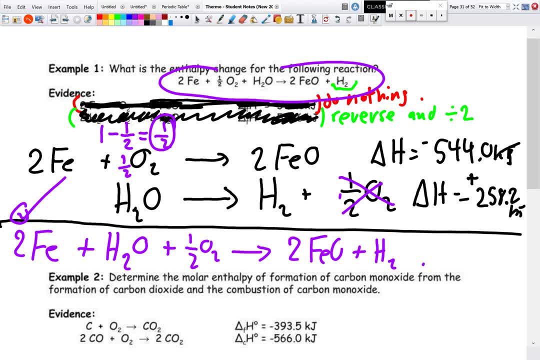 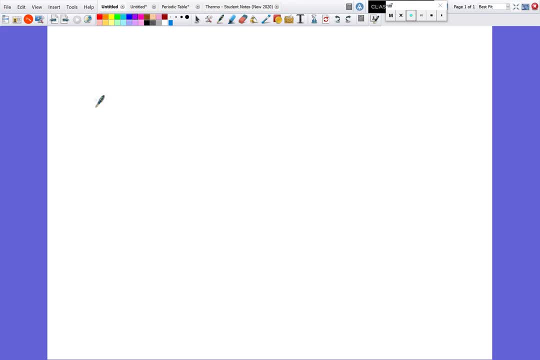 We have delta H. What we do here, delta H is equal to. We have two values right here, So if you remember, I'm just going to pull up something over here- We had delta H is equal to the sum of the enthalpy changes, right? 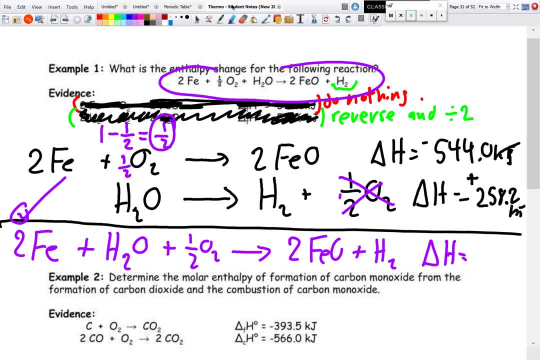 So that just means when we go back and look, we have a negative 544.0 and a positive 258.2 kilojoules. So what we're going to do is add those together. Now. you don't need to show this step. 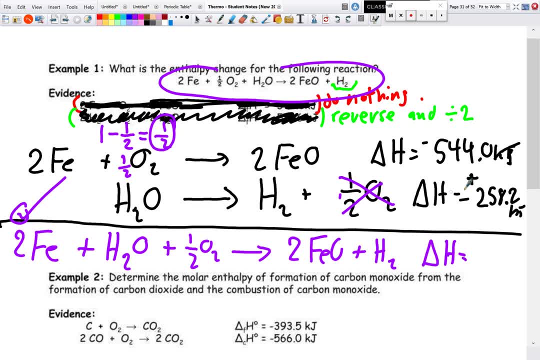 If you have them, Oh sorry, Sorry. If you have them lined up like this, you can just add them together and write your number down here, Right, But I'm just going to show you how that looks like when you add them up. 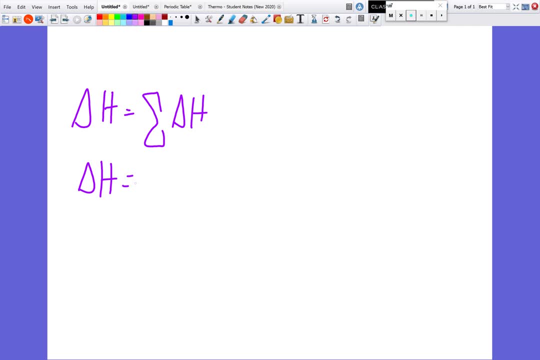 So we add them up: delta H for that reaction. We had our negative 544.0 kilojoules. We add this to our positive 258.2 kilojoules, Negative 258.2 kilojoules And our net enthalpy change is negative 258.2 kilojoules. 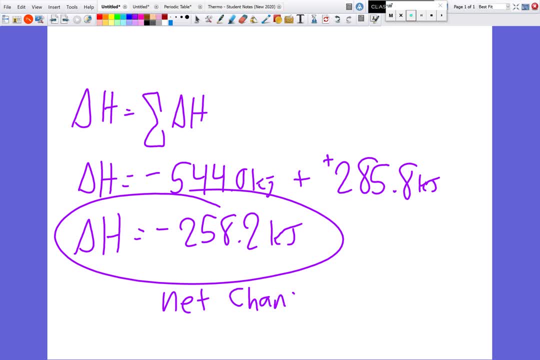 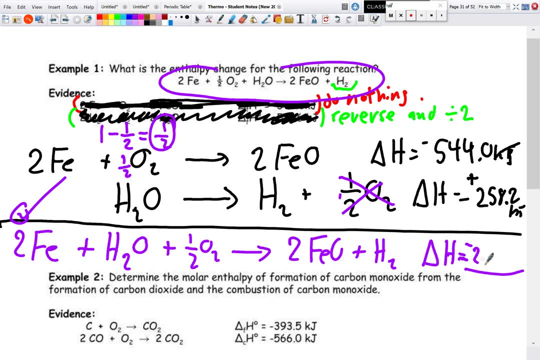 And this is our net change. So we take that number and we bring it over here to a negative 258.2 kilojoules. Yeah, 0.2.. I started running out a little bit of space right there, But that is how we find the enthalpy change for our unknown. 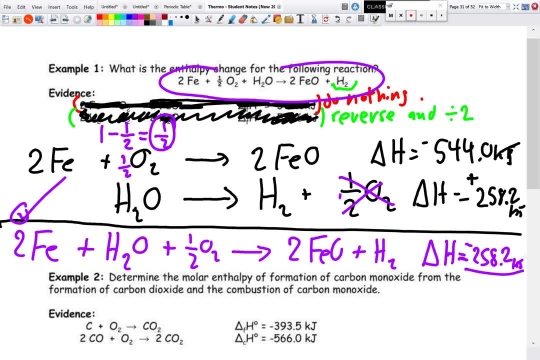 Now I know that seemed like a lot to kind of get tossed at you in the one go. That's why we're going to look at our second example And then hopefully by the third you'll be able to take it and kind of run with it once. 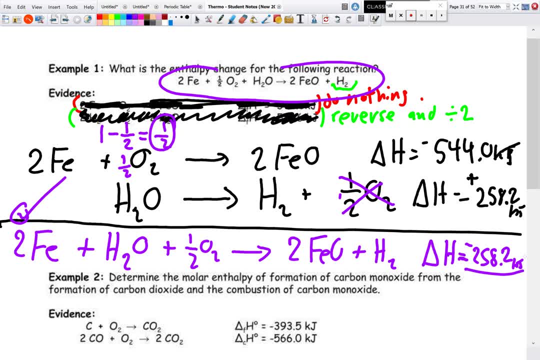 we get going. And then the fourth as well. So our second example that we're going to look at: Okay, So this is more, I guess, realistic of what I expect you to be able to solve, And the reason for that is when you look at reading it, it just says: determine first. 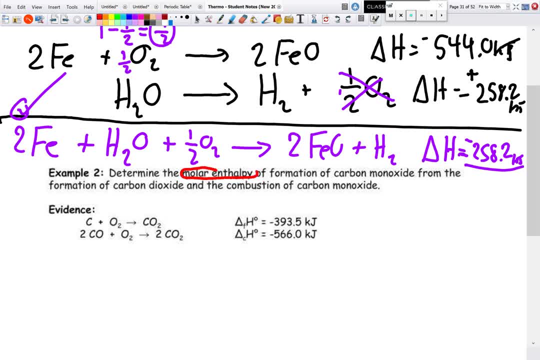 of all- I'm going to point this out- it says molar enthalpy, not just enthalpy change. So determine the molar enthalpy for the formation of carbon monoxide And we'll notice that there's no net. 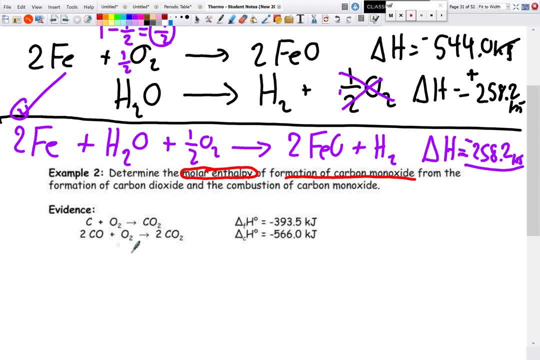 We're just given the evidence. So we have the formation of carbon dioxide and the combustion of carbon monoxide. Okay, So this is more realistic because you need to be able to provide your own net equation. So the net equation, the formation of carbon monoxide, we got carbon plus oxygen producing. 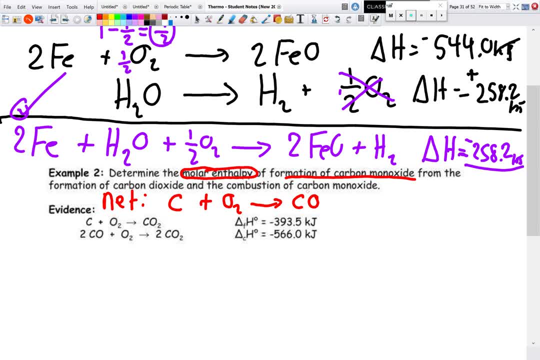 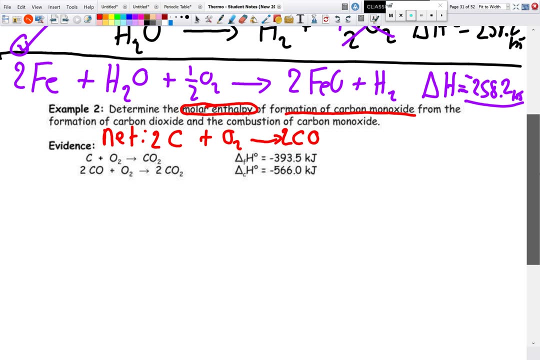 carbon monoxide. Now you do need to balance these as well. So you can use a fraction in front of oxygen, or you can just go two and two, and that works. It doesn't really matter what way you do to balance it. Now, if that is my net equation, now I'm going to start manipulating. 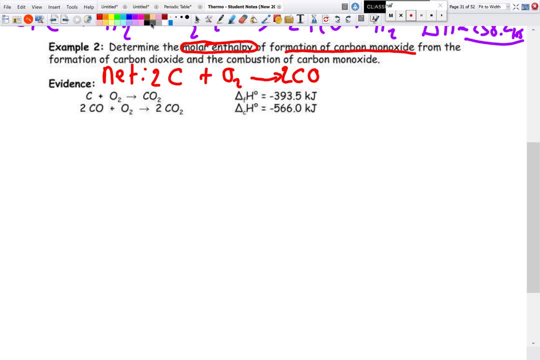 Okay, So same thing as before. You want to try to find those unique compounds that only show up in one equation and also shows up in your net. So for our first example here, if I look at carbon, I need two carbons as a reactant. 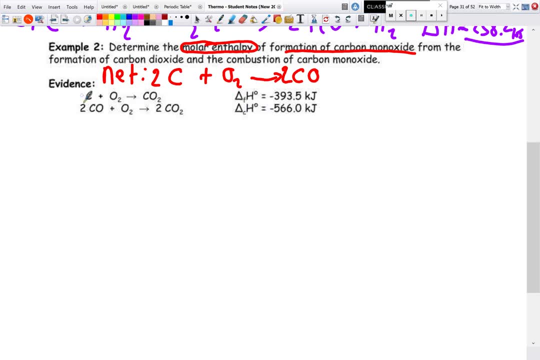 And carbon only shows up in this equation right here. my first one. But the coefficient is wrong. So we'll notice it's on the same side. So it's a reactant here and a reactant here which we need, but the coefficient's off. 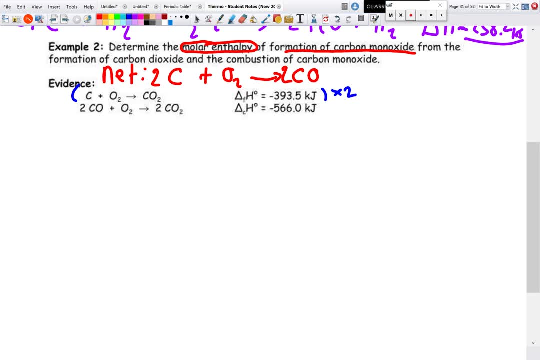 So I need to take this equation and multiply it by two. Okay, Multiply by two to get the correct coefficient in front. So that means I'm left with 2C plus 2O2, producing 2CO2.. And my delta H is also doubled to a negative 787.0 kilojoules. 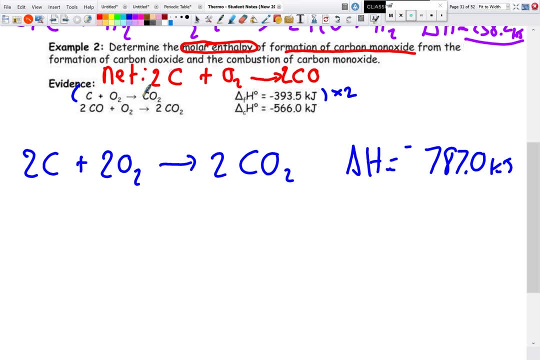 Now for my second equation. we'll notice that our unique compound That's going to show up is definitely carbon monoxide, because we have carbon monoxide up here in my net. Now, when we notice the coefficient two carbon monoxide, two carbon monoxide. 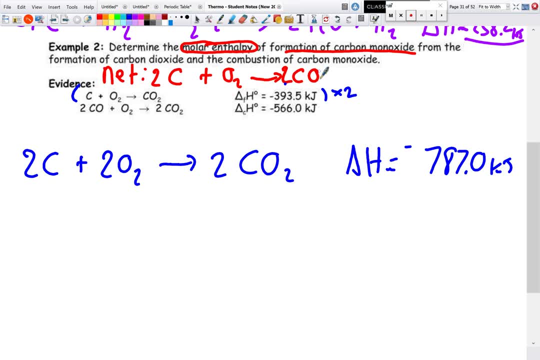 So the coefficient's fine, but the position of it or the side, is wrong, because here is a reactant, here it is a product. So I need to take this and reverse it. So when I reverse it, I'm going to rewrite my equation. 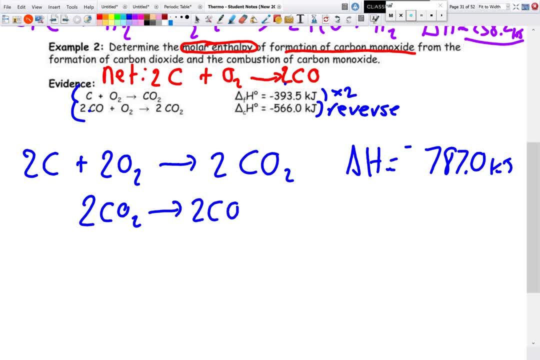 So 2CO2, arrow 2CO2.. Okay, 2CO plus O2, and delta H is reversed as well, So it is a positive this time. 566.0 kilojoules. Now add them together for my net. 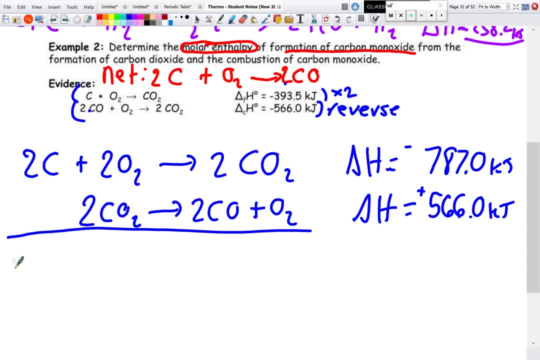 Just like before, we're going to look for things canceling out or things adding together. So let's look at carbon. We have carbon over here as a reactant. There's no other carbon anywhere in my two equations, So that means carbon is going to come down here. 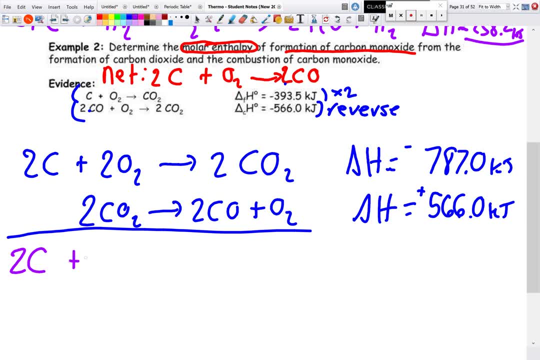 I'm scathed So I can write 2C plus Next, if I look at my oxygen, So same thing as last time. we see 2O2 as a reactant and just O2 as a product. Now there's one here and two here. 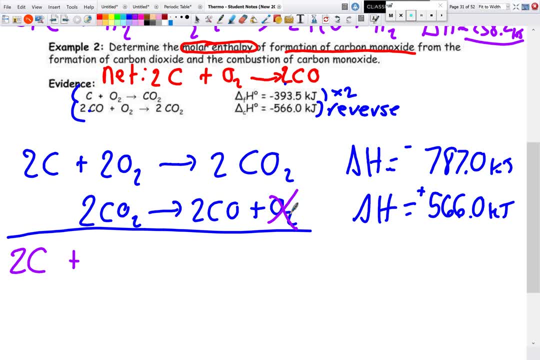 So obviously one is the lower number. So all of these auctions are going to cancel out. Now to figure out the new coefficient for auction, I do a little bit of math. I got two right, Because two here minus well, coefficient from the auction over here is one. 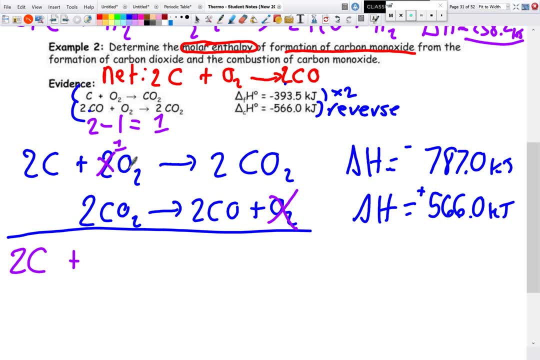 So I'm left with a one. So that means this is going to cancel out. This is going to cancel out to one: 1O2.. Now, remember, you don't need to write out the one, So we can just erase that and that'll be fine. 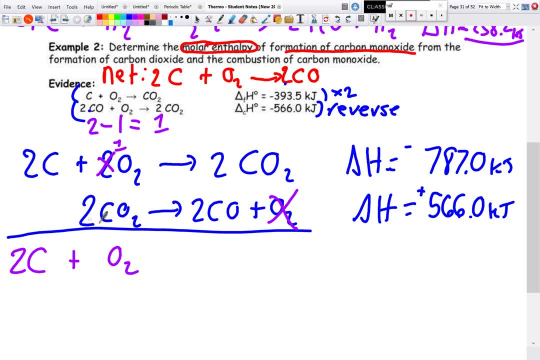 Now the last one we're going to look at is my CO2.. Now notice, on this side, right here, I have two CO2 as a reactant and two CO2 as a product, Because these are on opposite sides of the equation and their coefficients match exactly. 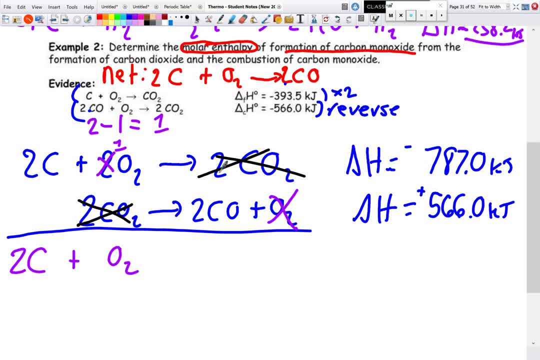 they cancel out completely. And, last but not least, for our products, the only thing that's left is two CO. And finally, last but not least, we're just going to add our delta H's together. Now, this one. if you want to show the math for this, you can, but you don't really need. 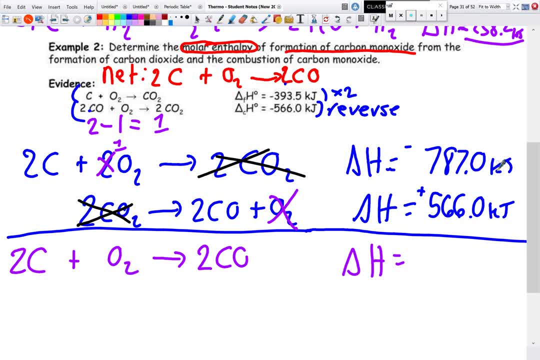 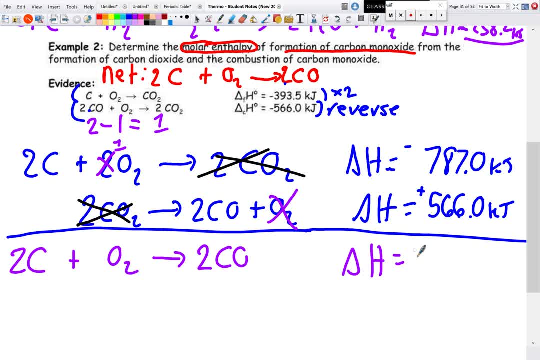 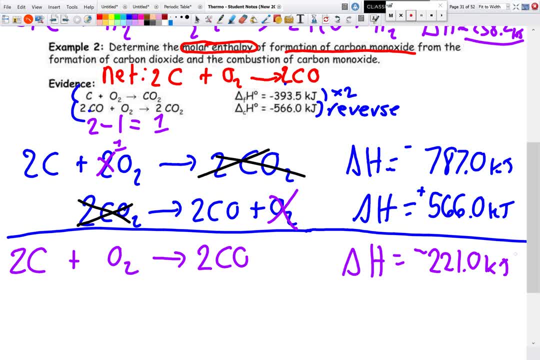 Now, whenever you write out a question, always ask yourself: the last question is: did I answer the question Now? as I pointed out when we first started this one, we want molar enthalpy. This is enthalpy change. it's not molar enthalpy. 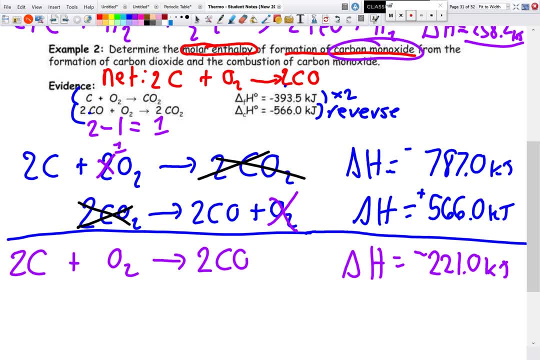 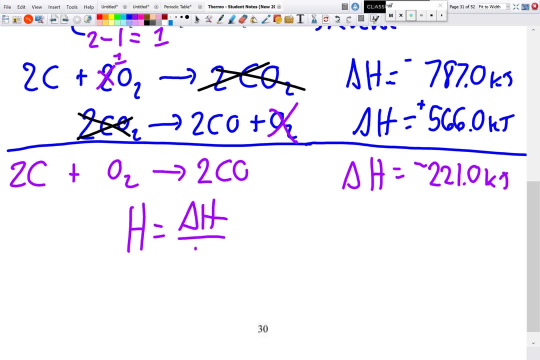 So, and I want the molar enthalpy for carbon monoxide, So I'm not done, I need to go. molar enthalpy is equal to the change in enthalpy over number of moles. Now this is going to be for CO, so the number of moles also needs to be for CO. 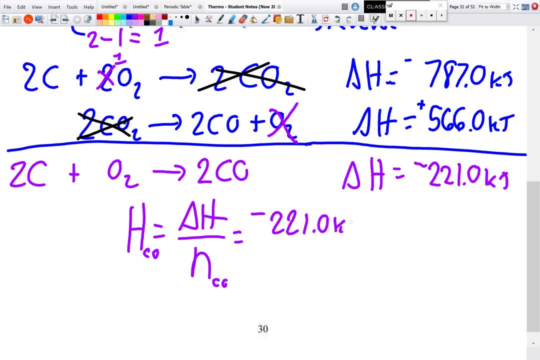 So that means I take my negative 2 to 1.0 kilojoules and I divide by the coefficient in front of CO, which is 2 moles, And we're left with negative 1.10.5 kilojoules per mole. 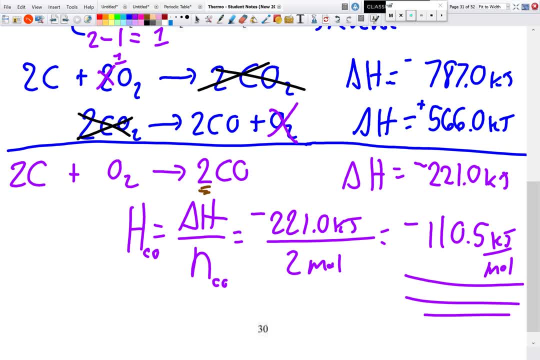 And that is my final answer, because I know I have the correct units. So that, of course, is Hess's Law. Now, once again, this is more of a realistic example, just because we weren't given the equation first. Now, on the next page, it does say, once again, a more realistic situation. 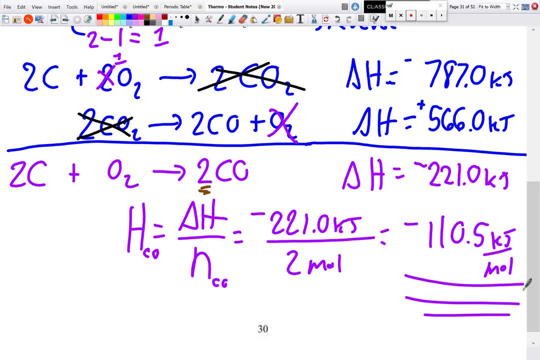 And by realistic it means lab. So if you're ever doing this and you're doing research or anything like that, there's a chance that all the given equations aren't going to be nice and neat and ready for you. You need to scour some books, scour the internet. 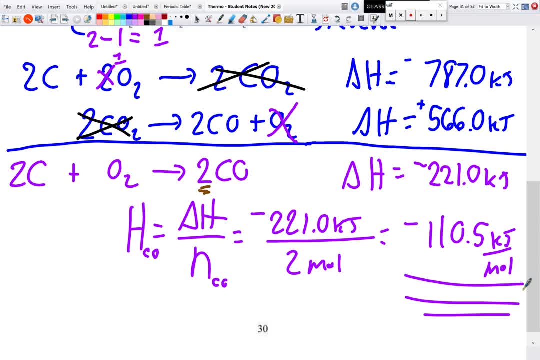 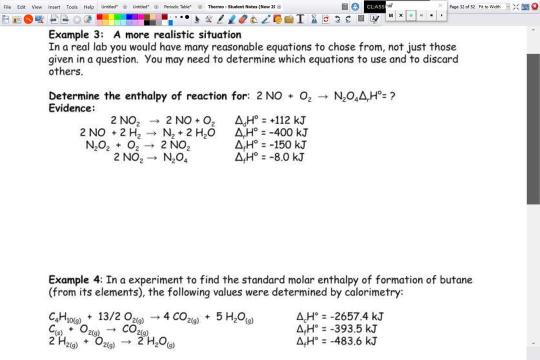 and try to find equations that you can use to manipulate in order to solve for Hess's Law. So let's look at them Now. I'm only going to help you start this question, and then I want you guys to try to finish it. 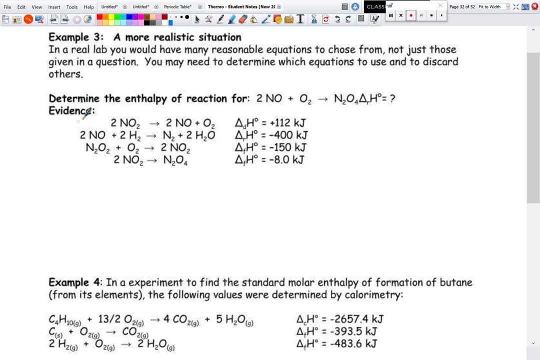 And then I'll have the answer up now in a little bit. So if you're ever given one like this, so this one. here we have four different equations. I know what you're thinking is like: oh my god, I have to use all four. 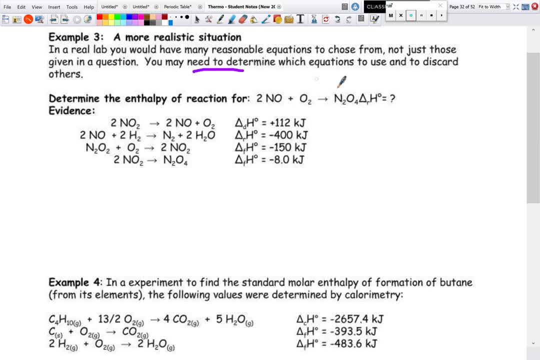 Well, it says right here we can determine if we can use or discard information. So when we look at this, delta H should be spaced out a lot further over here. So this is our net equation that we're looking at. 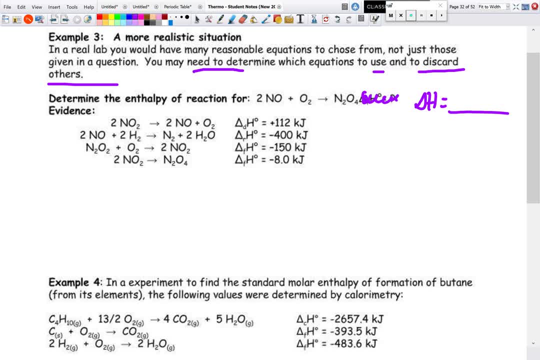 So we got two nitrogen monoxide plus one. oxygen produces one Dynitrogen tetraoxide. Now, looking at this same thing I always like to look at you know unique molecules, so I see NO, So nitrogen monoxide I know here. 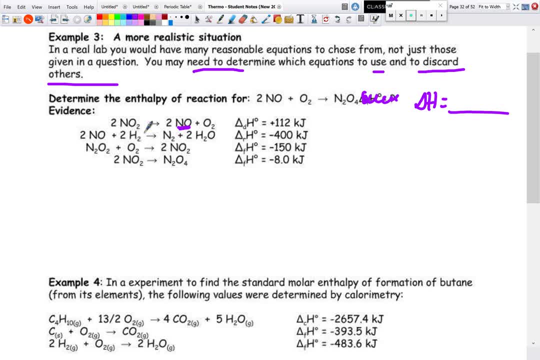 So therefore, I can kind of piece together that I might need to use equation one, But you are going to notice, okay, nitrogen monoxide, it shows up in equation two. So when you're into this situation, start trying to think ahead of the game and be like okay. 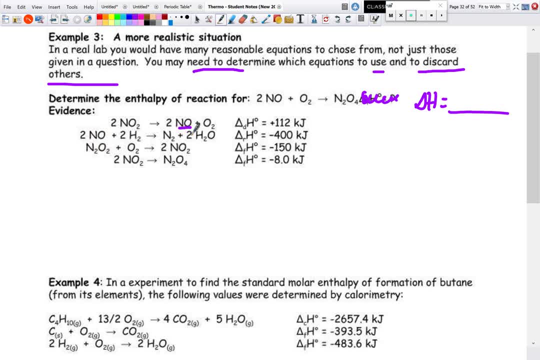 if nitrogen monoxide shows up in equation two, then I'm going to need to use equation three. So if nitrogen monoxide shows up here and notice how nitrogen dioxide does not show up in our net, is there an equation I can cancel out nitrogen dioxide? 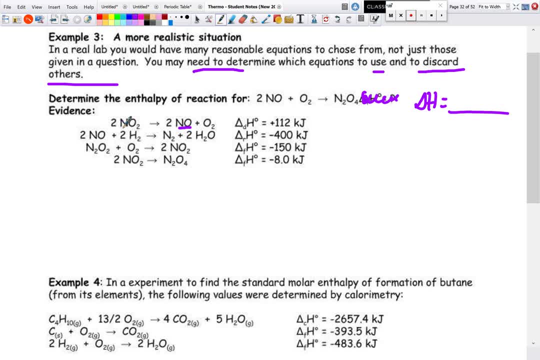 You're like: oh, this one right here, So I can potentially use a combination of equation one and equation four, right? I'm just thinking ahead Now. if I use equation two, right, and I use this for nitrogen monoxide. 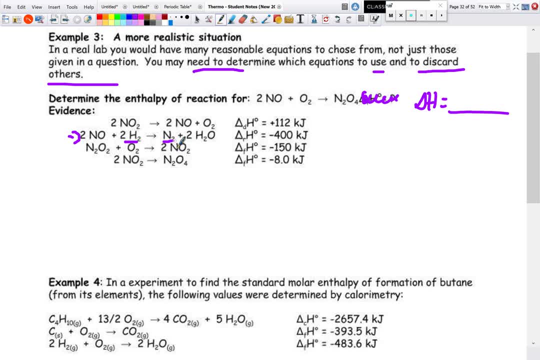 notice how we have hydrogen nitrogen and Y. So if you use this equation, you're going to bring hydrogen nitrogen and water into our net equation with no way to cancel it. So if you're offended with that, that means you're going to take this equation. 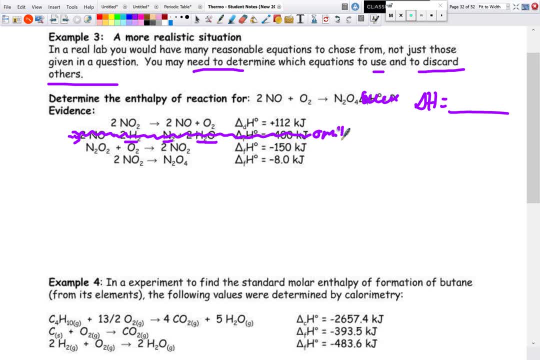 take it and omit, And that is the only way to answer this question. all right, Now there's going to be one more equation you must omit. So this right here, you're only going to use two equations. So, looking at that information, so the same logic I just applied to cancel out this one. 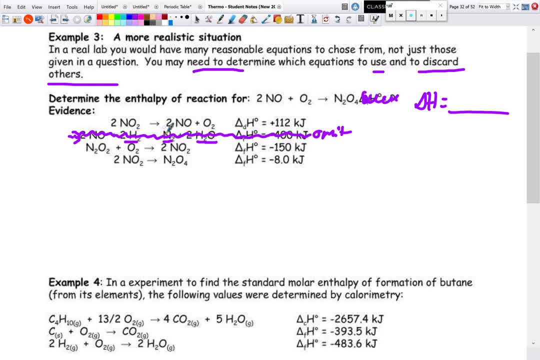 because I knew I would not be able to cancel out hydrogen and nitrogen if I used it. see if you can find that next equation, And when you do, you should get an answer of delta H is equal to negative one, So that's going to be 20 kilojoules, all right. 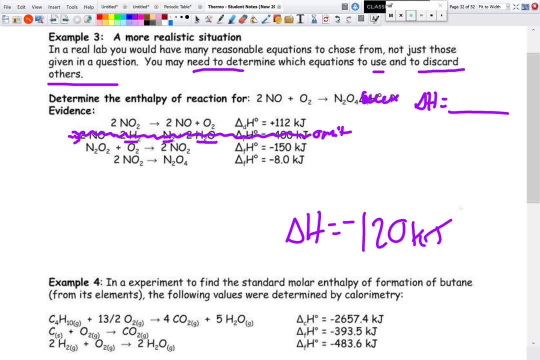 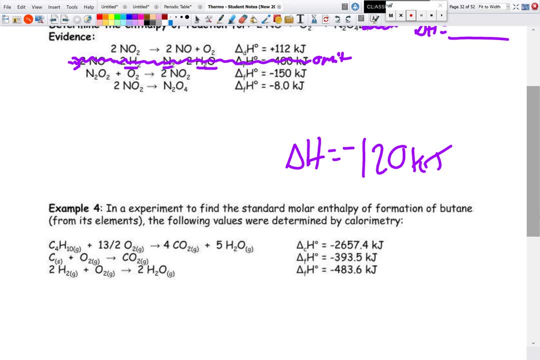 But you still need to make sure that you get this answer by manipulating the only two equations And, last but not least, when you guys just write this out on the side, just so you know what you do. if you do experiment or example four- sorry correctly, you will notice that no equation is given. 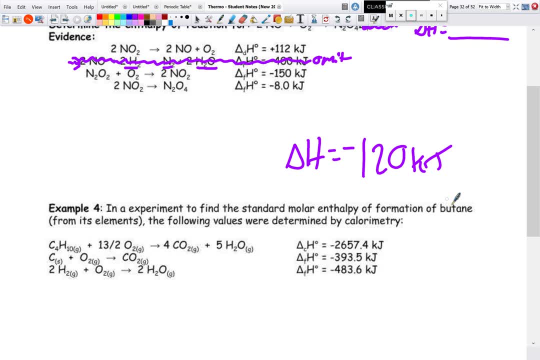 So you do need to figure out the standard molar anti-formation butane, and butane is C4H10.. You should get your answer. So H should be negative: 125.6 kilojoules per mole, hopefully. if you do that one correctly, all right. 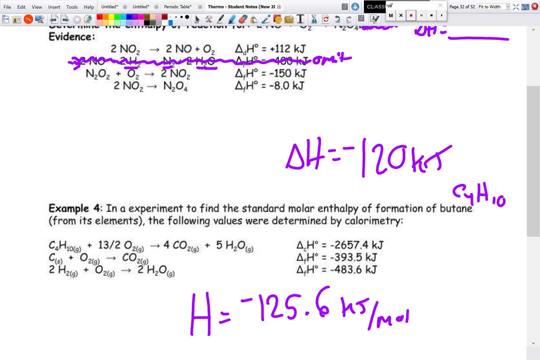 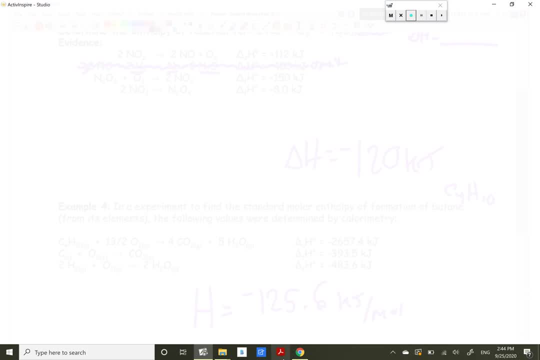 So try those, see if you can get those answers. If you don't, definitely make sure to contact me, just so we can try to figure something out Now on Google Classroom as well. so I'm just going to fire this up here now in a sec. 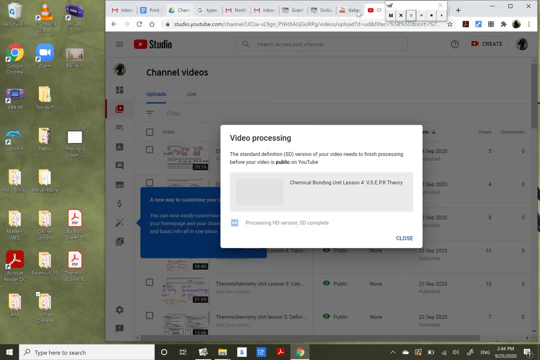 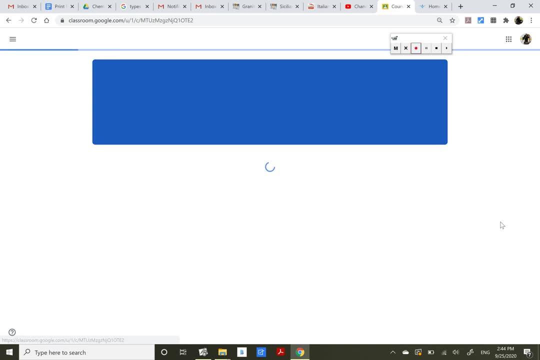 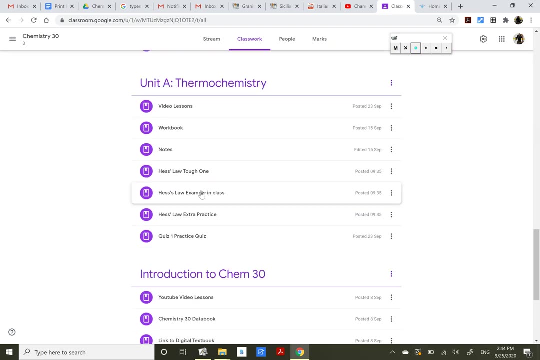 Oops, you don't need to worry about that. So on Google Classroom for our. oh, this is Chem 20,, Chem 30,. we will notice that I just uploaded in your classwork some stuff with Hess's Law. Hess's Law- a tough one. Hess's Law- example in class. and Hess's Law practice- extra practice. 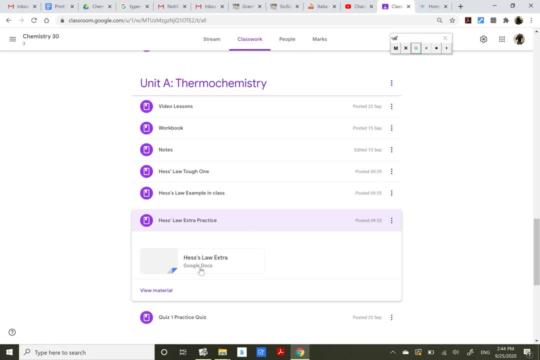 So this here is once you complete your workbook. if you just need five more, just a little more practice, open up this one. It has the answers with it. But don't worry, This is the one I passed out in class. 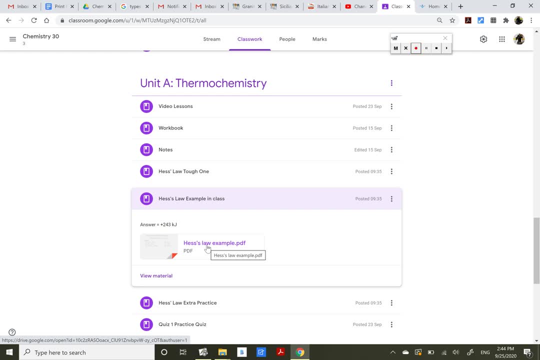 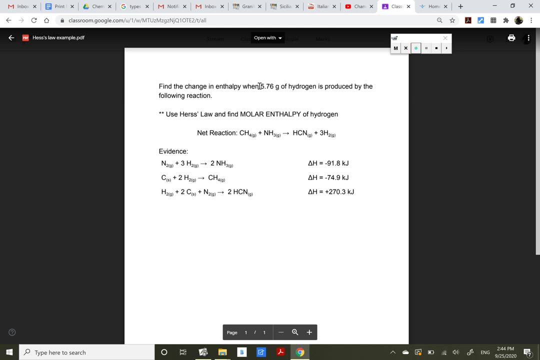 The answer is right here. Now, with this one, this is more of a typical type of example that you're going to get, because you need to use Hess's Law to figure out this, but you also need to figure out the molar enthalpy for hydrogen, because it's basically a two-stepper right. 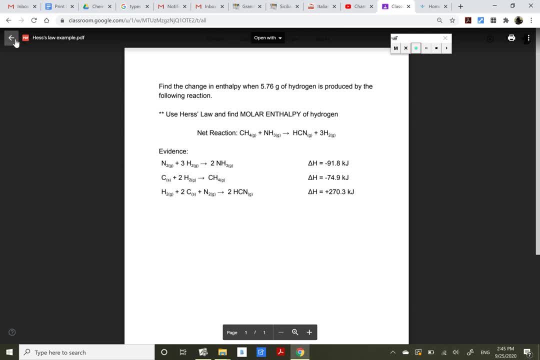 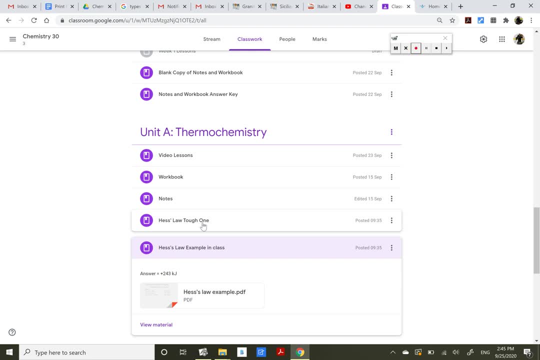 So please, please, please, try this one and see if you can get the answer. If you can't, once again let me know. The answer is right here. so you should get a positive 243 kilojoules. And finally, the tough one. 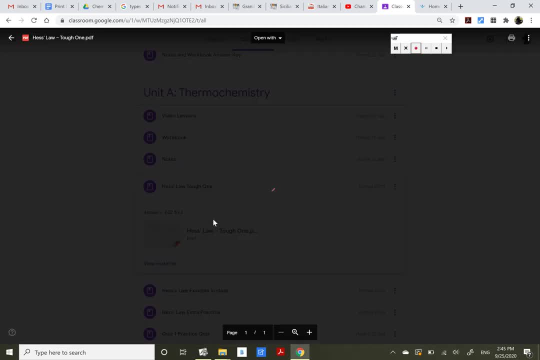 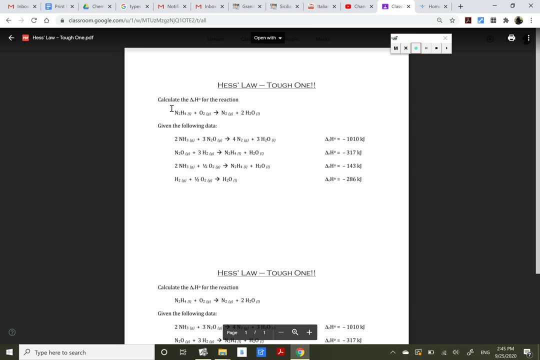 Now, once again, I have the answer right here. This is the one that this is the toughest one I can ever find, and you will not get one like this on a diploma. It's the exact same one, written twice. This is kind of one that, if you're really confident with it and you want to test your abilities, try this one right.